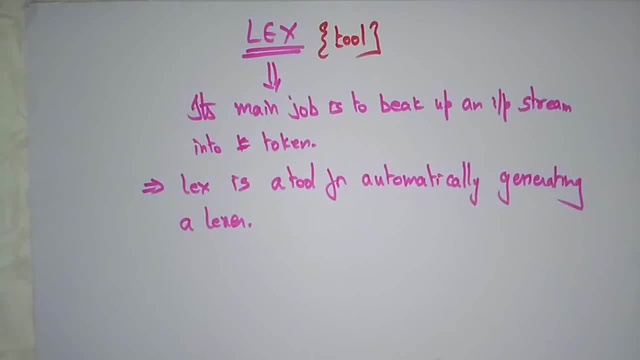 so this lex is a tool for automatically generating a lexer. so how it is going to be generated, how this lex is going to support the lexical analyzer to convert the source to the target means. it's just convert the source program into series of tokens, but by using this lex tool, let's see. let's take the lex source code. 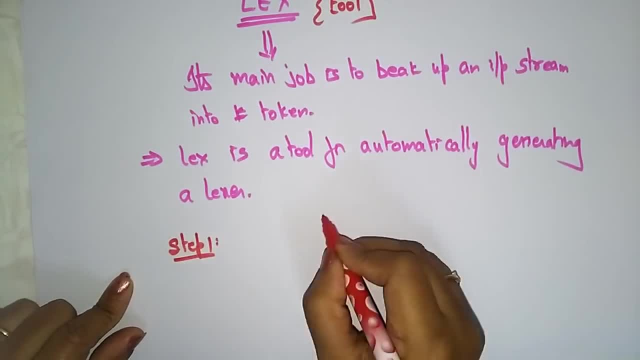 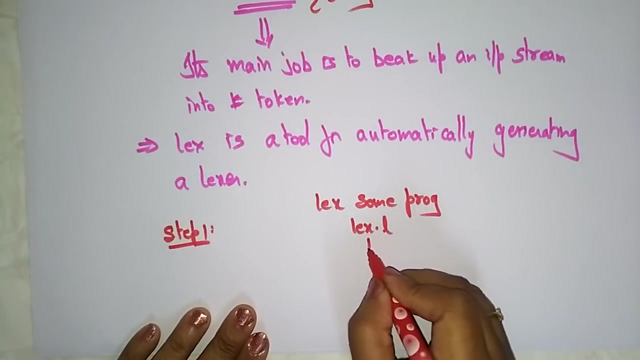 step one, let's take the lex source program. the lex source program is: let's take lex dot l, lex dot l, l dot l is the lex source program. so this source program is converted, sent to the lex compiler. So, with the help of the lex compiler, you will it generate an output as: 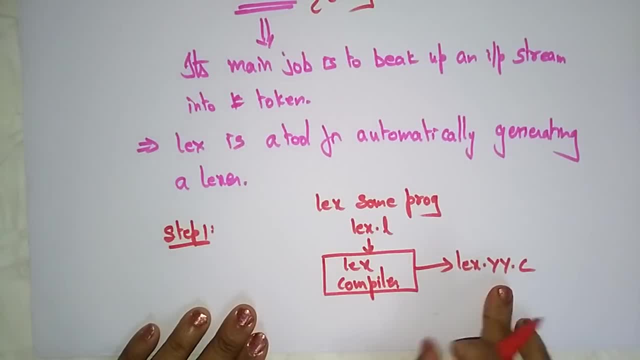 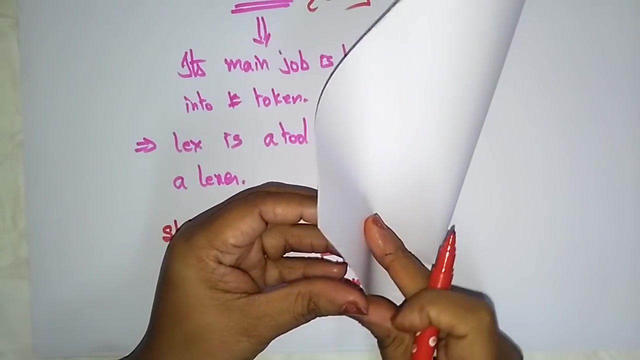 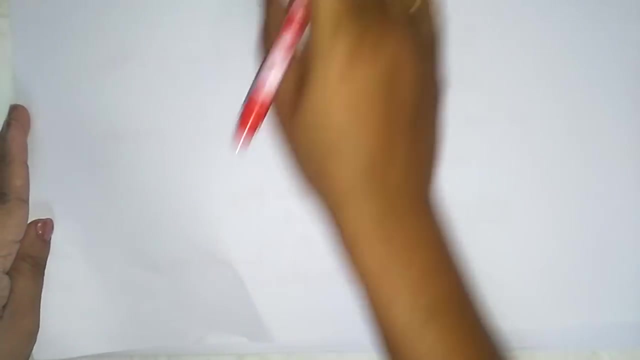 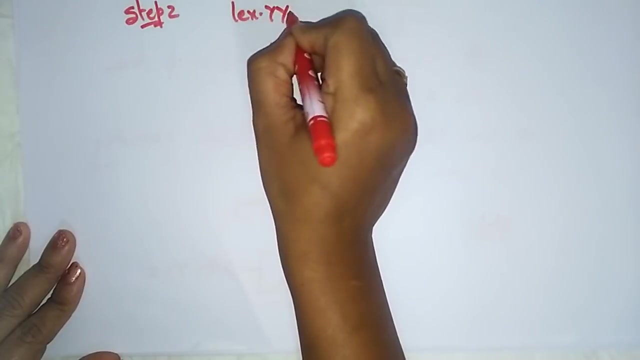 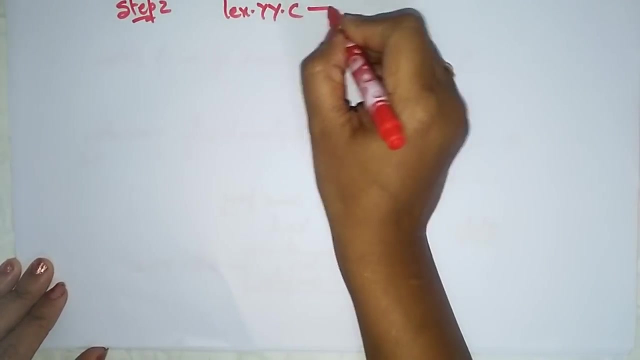 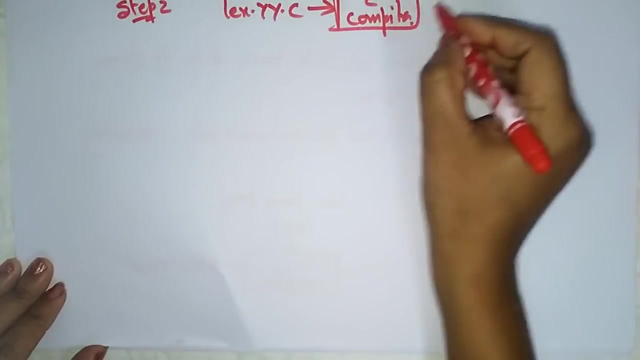 lexyyc. so, which is a input for the compiler. So the source program is converted into lexyyc, which is an input for the compiler. So in the step 2, this lexyyc, what is an output that we get from lex compiler? so this acts as an input to the c compiler and this c compiler is going to produce aout. 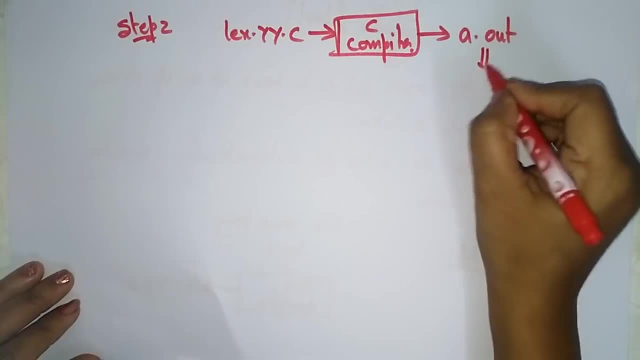 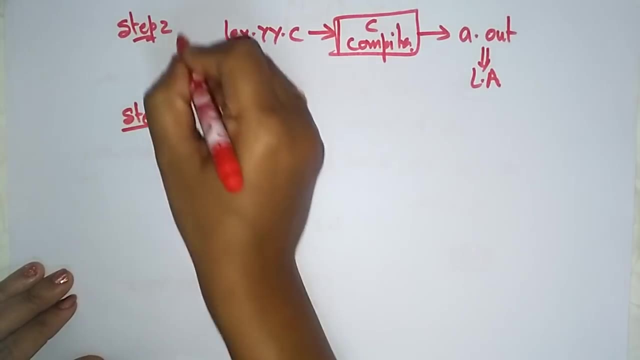 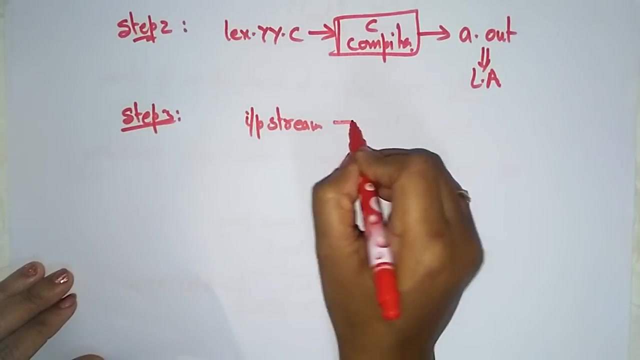 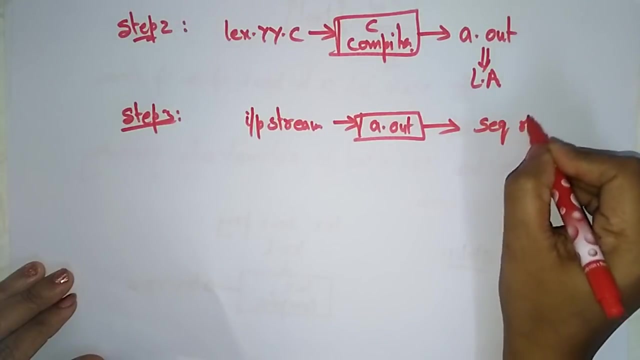 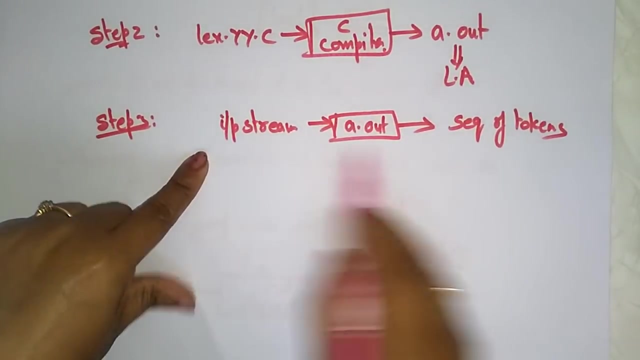 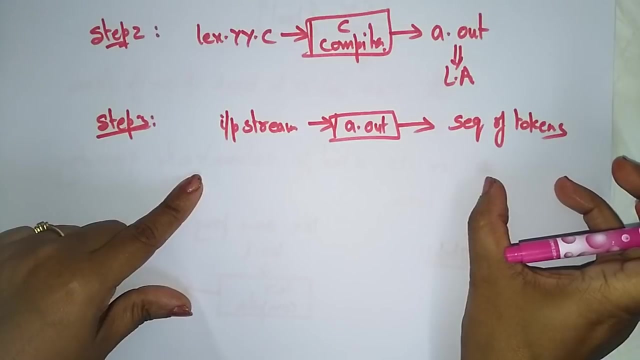 So aout or aexe, it's nothing but a lexical analyzer. Step 3. Input stream: whatever the lexical analyzer aout we get, that will be sent to the sequence- produce a sequence of tokens. Okay, so far we have just seen this thing: input stream, input stream, lexical analyzer produces a sequence of token. 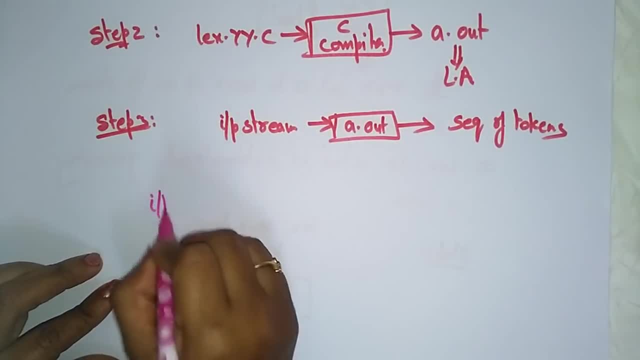 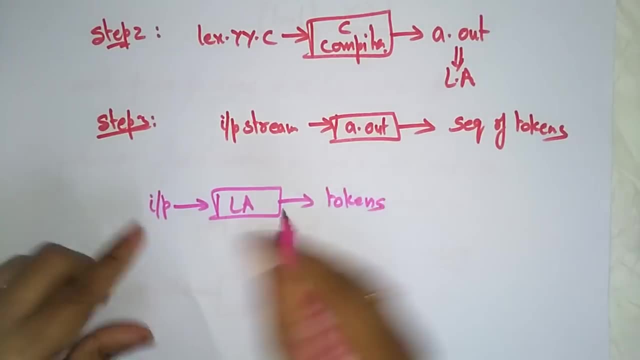 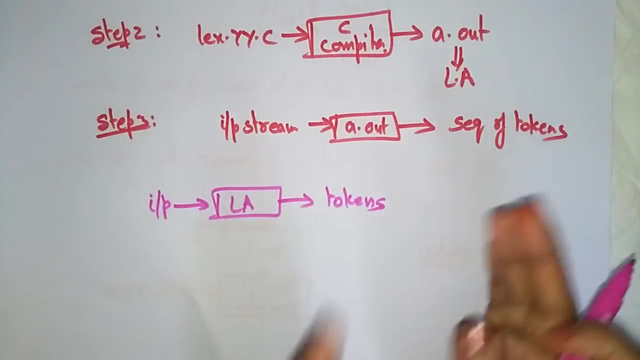 So how, internally, previously, what we are seeing? input lexical analyzer and it generated tokens. So input is a source code and the tokens. So here, what the lexical analyzer is doing. The lexical analyzer is taking the commands, It is taking the character one by one and it is going to be converted into, it is going to check what are the identifiers and what are the tokens and what are the lexemes, everything it is finding and it is producing a sequence of tokens to the as an output. 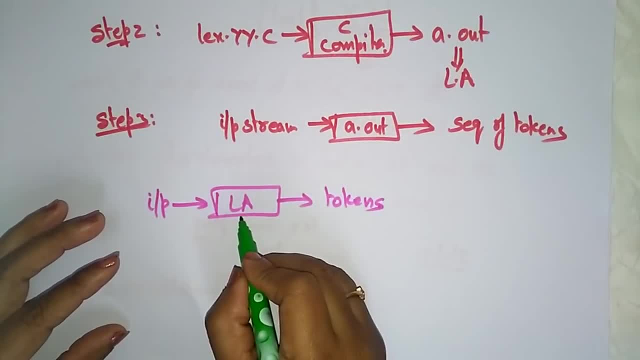 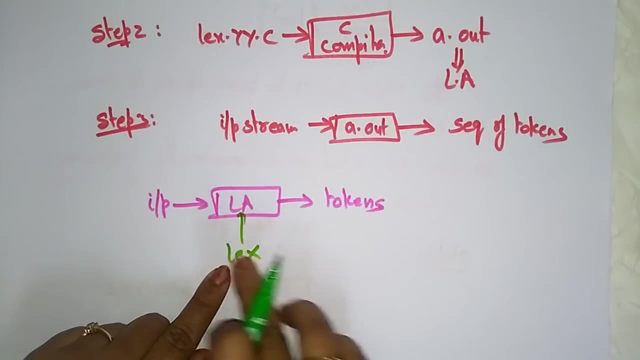 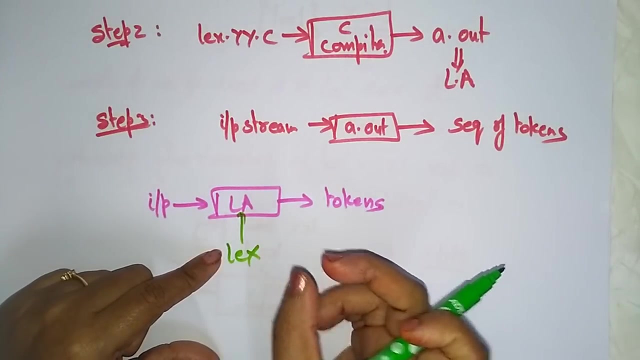 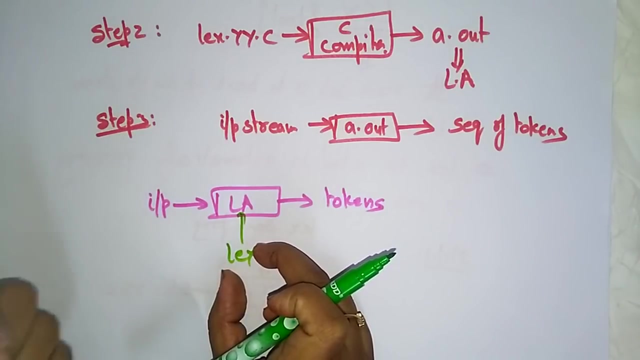 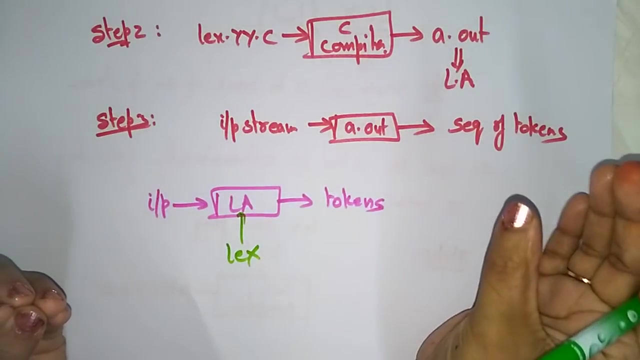 That it is doing, But with the help of the lex. okay, so here a lex will be there. So, with the help of the lex tool, it's automatically generating the tokens. Okay, how it is going to? So, it's with the help of the lex C compiler, with the help of the lex compiler. that lex compiler is already compiled, whatever the source program that is there. it's just taken the tokens and it is compiled, and it is with the help of the C compiler. it is producing exactly what the lexical analyzer wants. 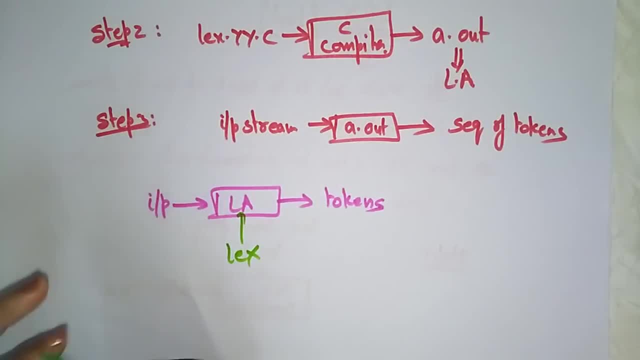 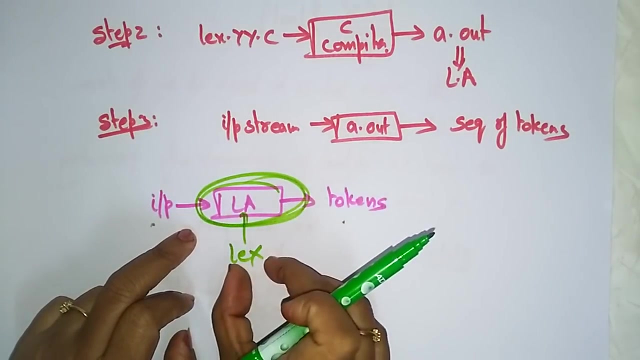 Okay, so don't be confused: Just input And we need an output as a tokens. So in between this there is so many operations of performing. Okay, so by skipping all those operations that are performed by the lexical analyzer, the lex tool is automatically generating what exactly the lexical analyzer wants. 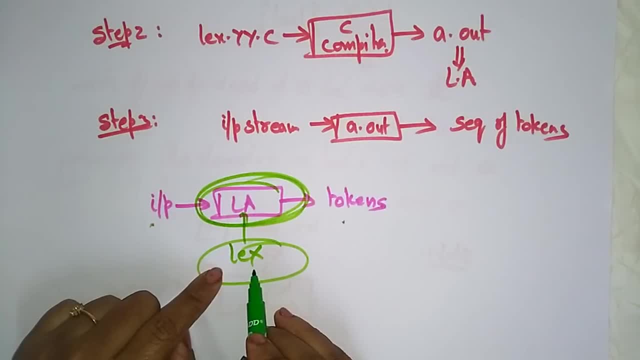 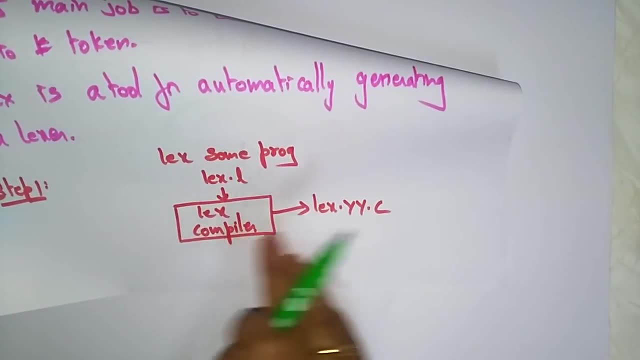 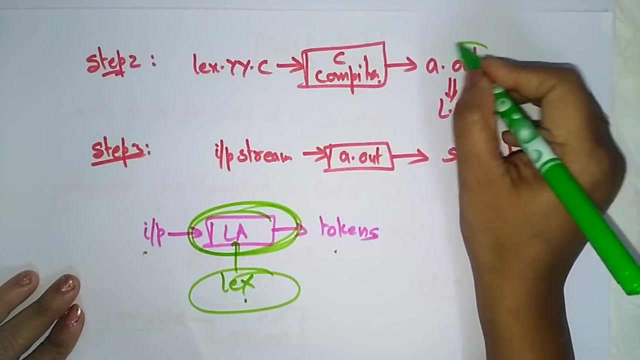 So everything will be done in the lex compiler. So what it is doing here, So it's a step one- It's just take the source program lexl and send to the lex compiler And it is generating one output. That output is again sending to the C compiler and it is producing what exactly the lexical analyzer wants. 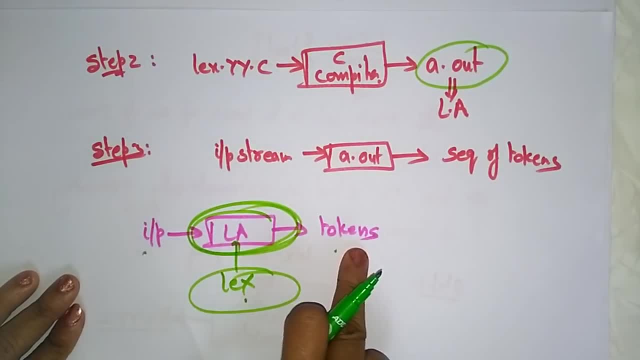 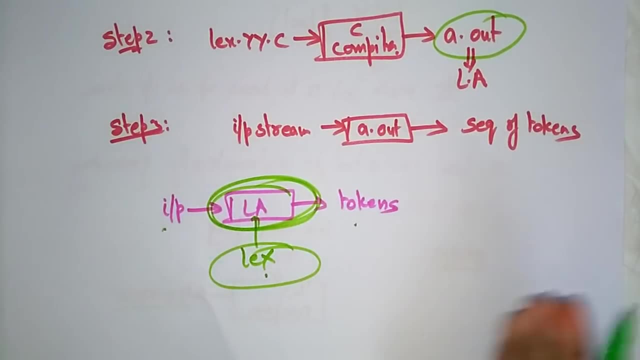 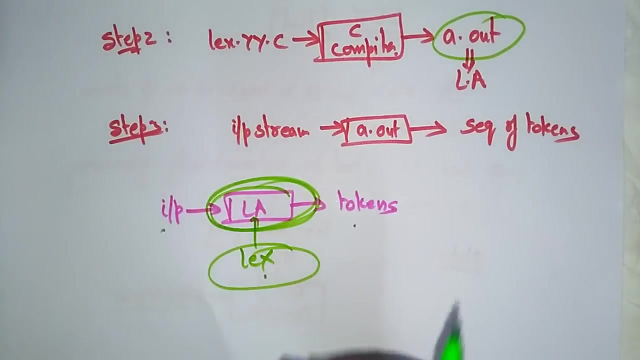 So that will be stored here and sends the sequence of tokens. Okay, so this input stream, whatever the input stream that it is getting, so that source code and relating information to that source code will be sent to the lexical analyzer. Okay, now let's start. 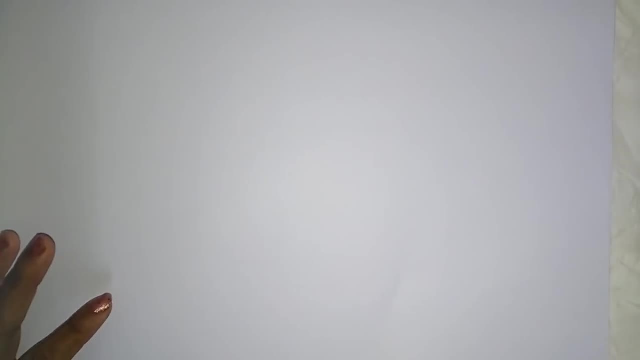 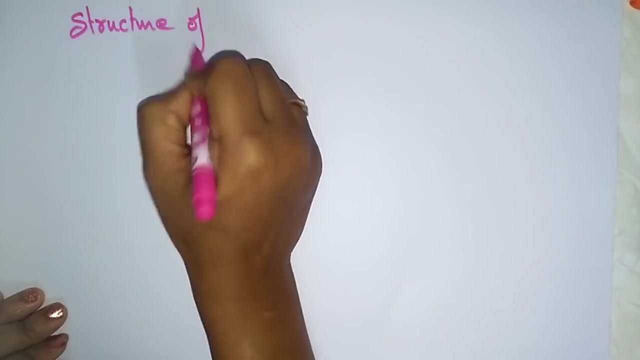 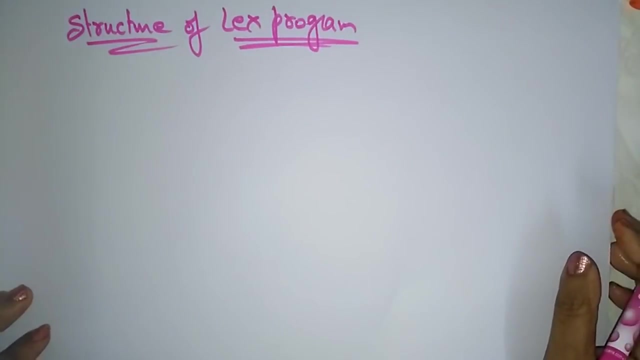 See the structure of lex program. structure of lex program. so don't be confused. The lex tool is only. it is a source program which supports with the. with the help of the input source code, it converted what exactly the lexical analyzer wants. Okay, So with the help of this tool, the lexical analyzer is going to generate tokens automatically. 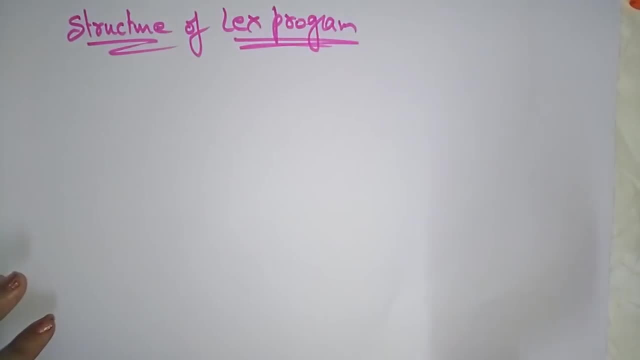 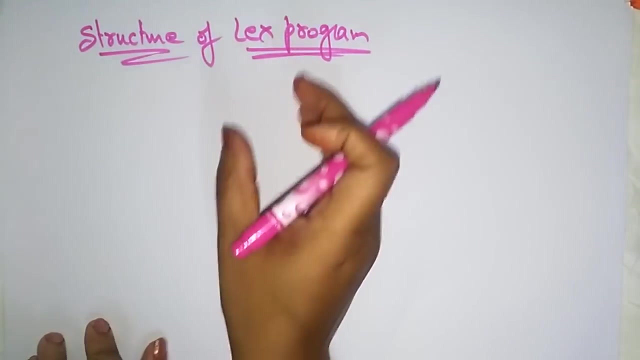 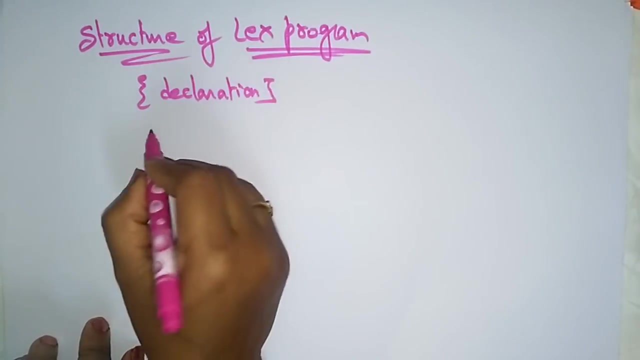 That is a main concept. with the help of the lex tool, The lexical analyzer is going to generate tokens automatically. So what is the structure of lex program? Declaration is a one section and the next section is the translation rules. So what is the structure of lex program? 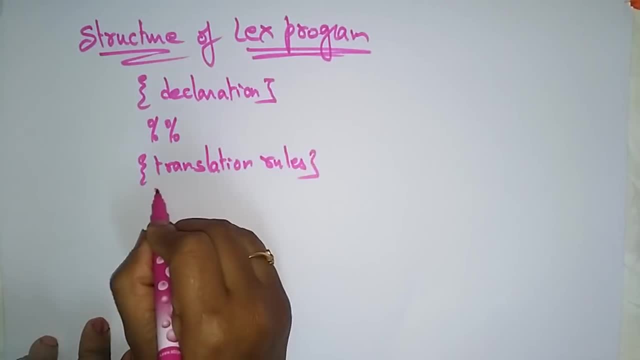 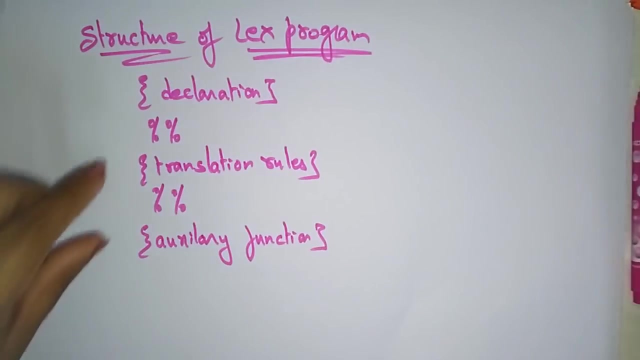 Declaration is a one section and the next section is the translation rules, Translation rules And the third section: total three sections will be there. So this third section is an optional one. So total three sections will be there. Okay, so the declarations section. 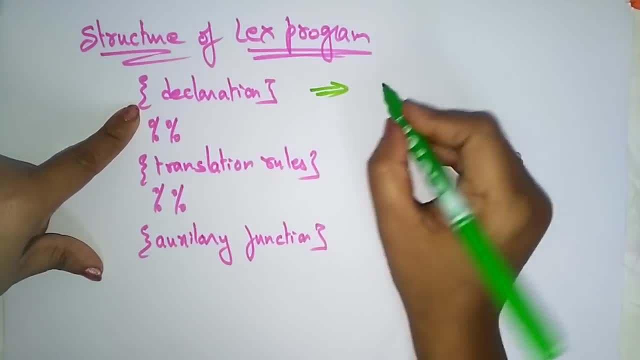 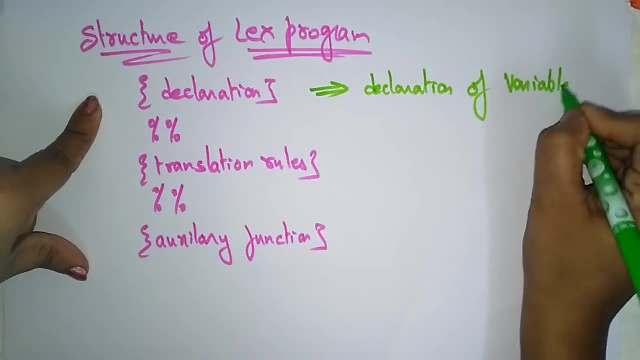 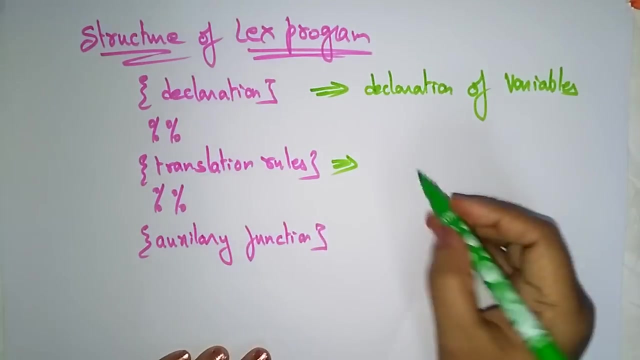 So what this declaration section consisting of? So it declares all the variables. Declaration of Variables: So it declares all the variables, variables and translation rules. the translation rules have the form of patterns, actions, like that. so, whatever the program that is, we are writing, uh, taking the input input stream, so that input stream. 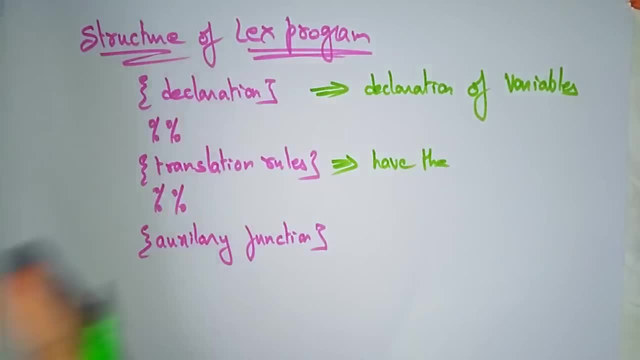 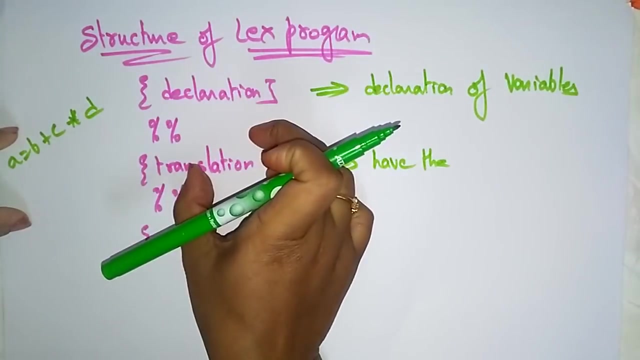 will be represented in the form of flex program, so that input stream whatever we are taking. let us take a is equal to b plus c into d. so this input uh stream is going to be converted into uh with the help of the lex program. so this is an input stream. let me take this is an input stream. 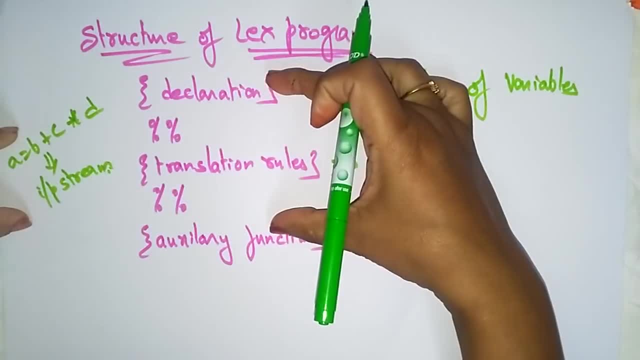 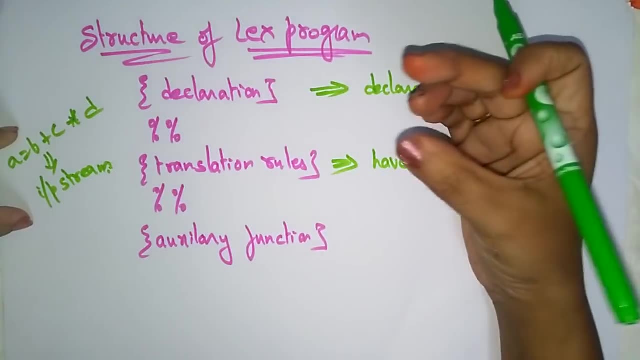 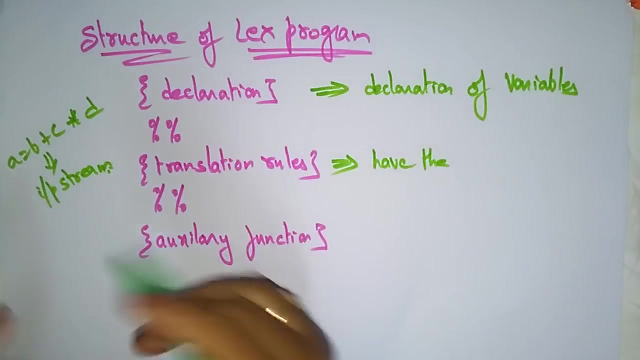 so this input stream is uh returning in the form of flex program. so if it, if we return in the form of flex program, then the lexical analyzer can easily understand what is, what are the tokens here and what are the uh, what is the operation it is going to be, uh performed, so everything will be understand.